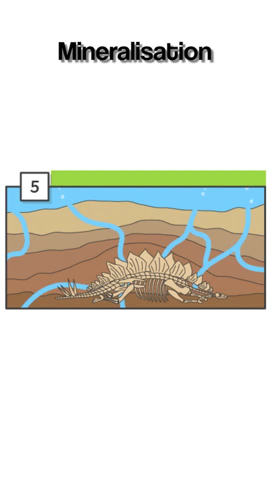 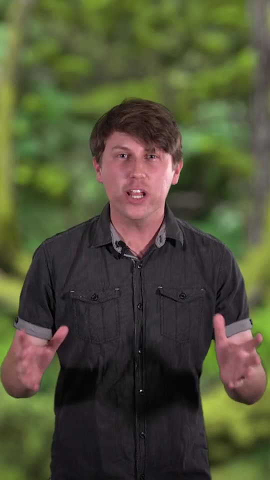 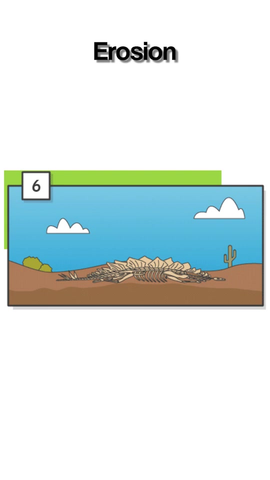 containing minerals which then seep inside the fossil material. The organic material is replaced with these minerals and becomes a fossil After millions of years. tectonic events such as earthquakes and mountain ranges rising and falling will push the rocks containing the fossil material back up near the earth's surface, just waiting to be dug up by paleontologists. Visit Prehistoric. Australia for more Closed captioning provided by the Amaraorg community. 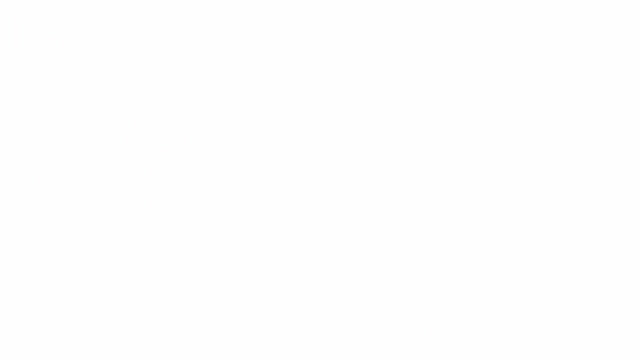 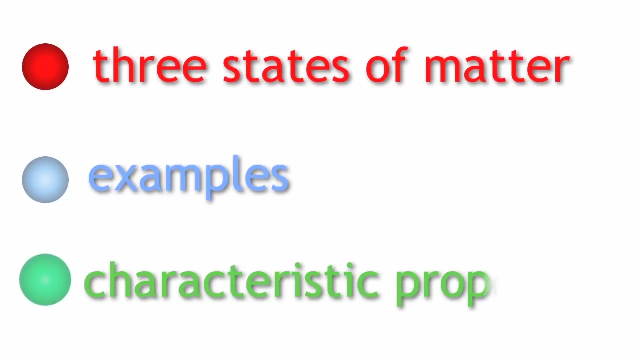 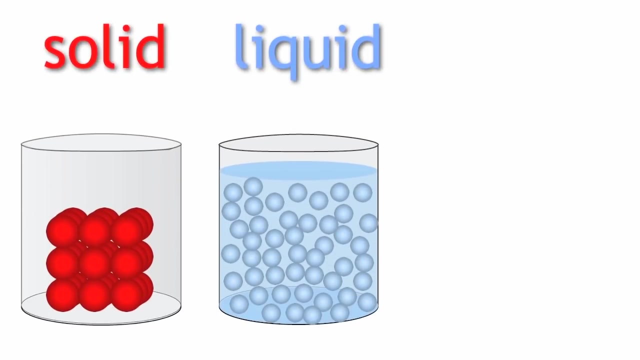 States of matter. In this video you are going to learn what the three states of matter are. some examples of each state of matter: the characteristic properties of the three states of matter. The three states of matter are solid, liquid and gas. Let us look at solids. 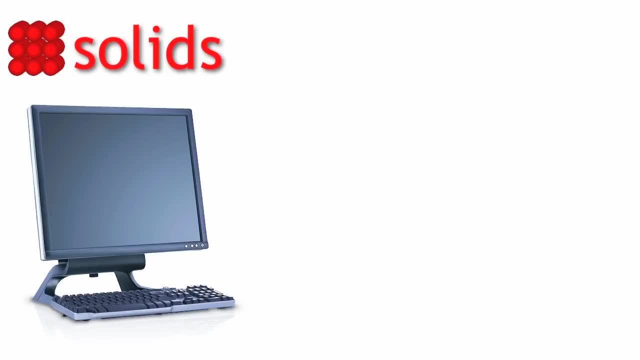 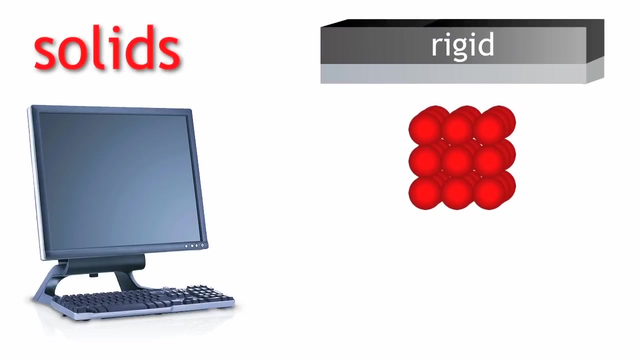 An example of a solid is your computer. The properties of solids depend on how the particles in solids are packed. In a solid, the particles are closely packed in fixed positions and cannot move anywhere. So solids are rigid, cannot be squashed or compressed, have a fixed shape and 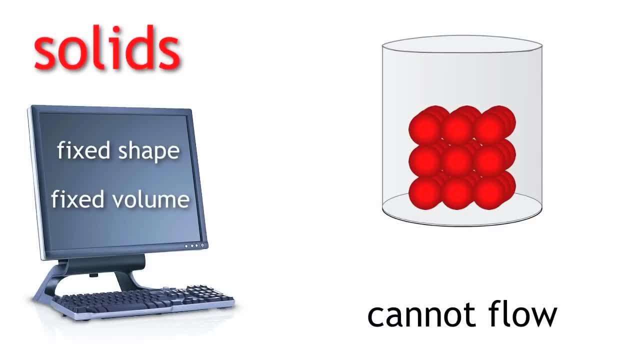 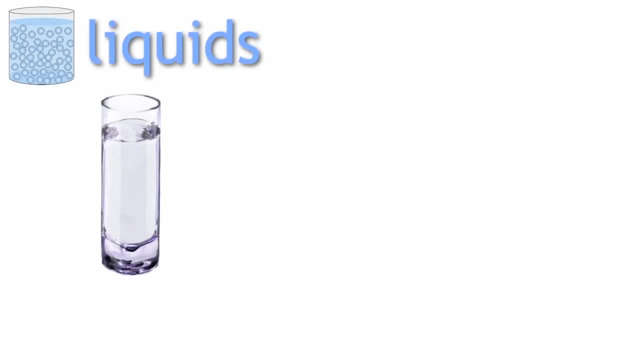 a fixed volume, They cannot flow. Now let us look at liquids. An example of a liquid is water. Just as with solids, the properties of liquids depend on how the particles in liquids are packed. In a liquid, the particles are again closely packed, but not as closely packed. 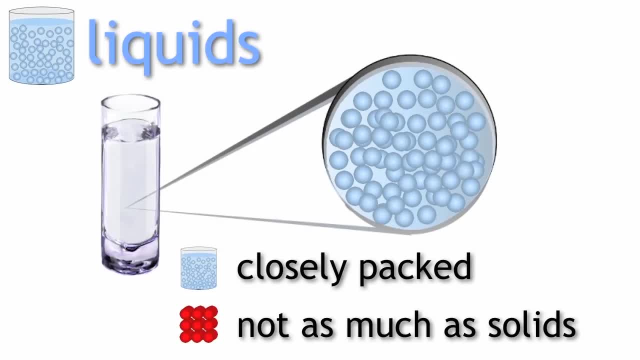 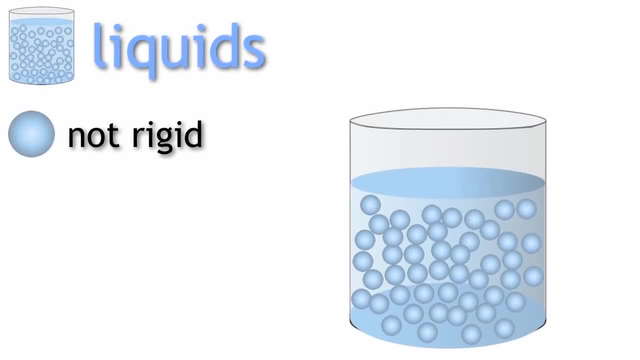 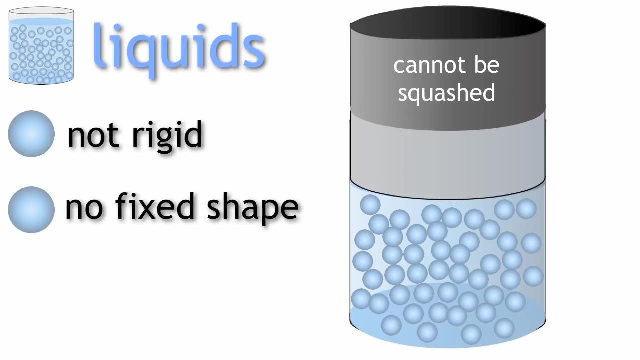 as in solids. So this means the particles in liquids can move around each other. So liquids are not rigid, but because their particles are closely packed, as in solids, they cannot be squashed or compressed. They do not have a fixed shape, but they do have a fixed volume. Beware with that one, as many students think that solids are rigid, but they are not. So let us look at solids. An example of a liquid is water, Just as with solids. the properties of liquids are rigid, but because their particles are quickly packed, they cannot be squashed. 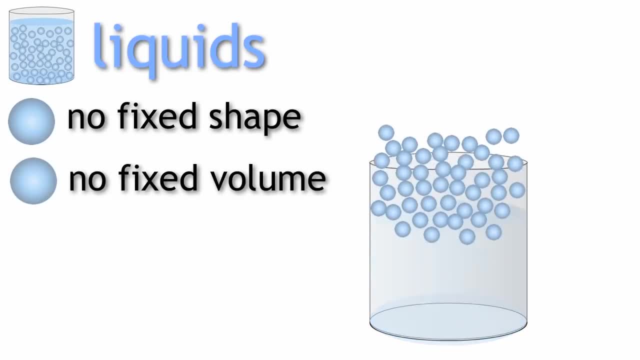 or compressed. They do not have a fixed shape, but they do have a fixed volume. So this is the law in a liquid. This is the role of the liquid in the case of solids and liquids. Here we have already discussed that solids are rigid, but they do not have a fixed shape.